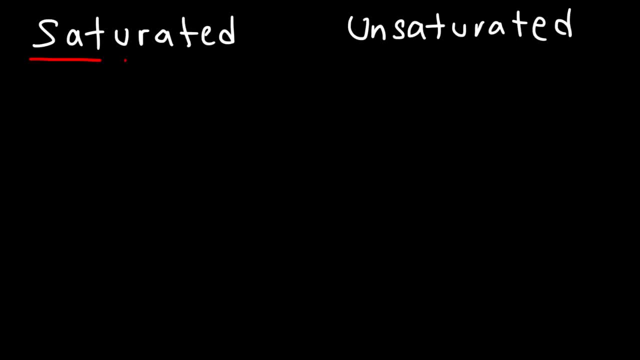 So what is the difference between a saturated hydrocarbon and an unsaturated hydrocarbon? Saturated hydrocarbons are basically alkanes. They're completely filled with hydrogen atoms. They have the maximum number of hydrogen atoms per carbon atom. So anytime you have an alkane. 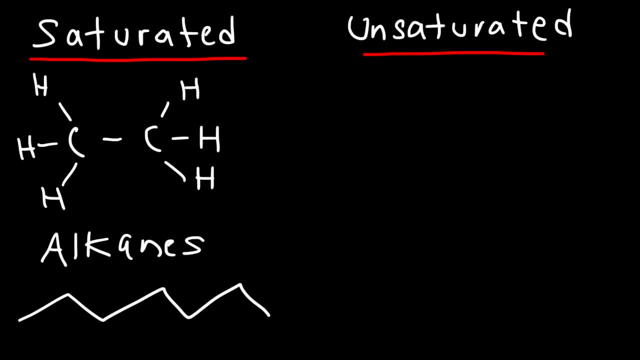 you have a saturated hydrocarbon. There are no double bonds, only just single bonds or sigma bonds. Now, unsaturated hydrocarbons include alkenes. whenever you have a carbon-carbon double bond, Alkynes- those are unsaturated, And even a benzene ring. that's another unsaturated hydrocarbon. 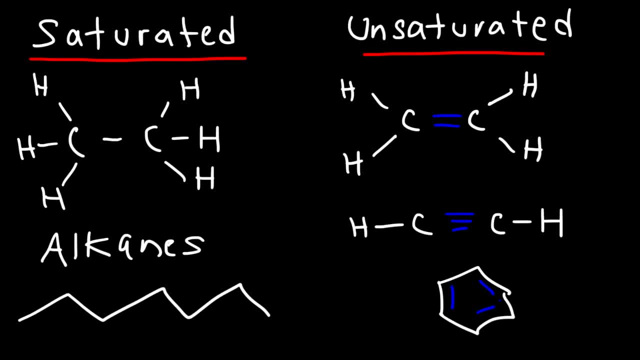 So anytime you have a pi bond. So if the molecule has any double bonds or triple bonds, it's an unsaturated hydrocarbon. If it only contains single bonds, then it's a saturated hydrocarbon. So make sure you understand that unsaturated hydrocarbons include alkenes, alkynes and 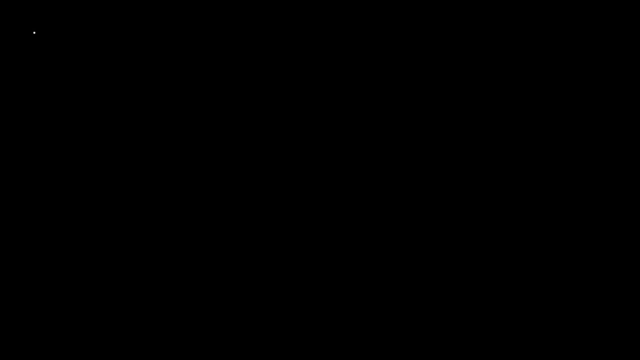 aromatic rings And only alkanes are saturated. Now let's talk about the alkanes, the saturated hydrocarbons. The general formula for an alkane is CnH2n plus 2.. So this is the general formula for an alkane. 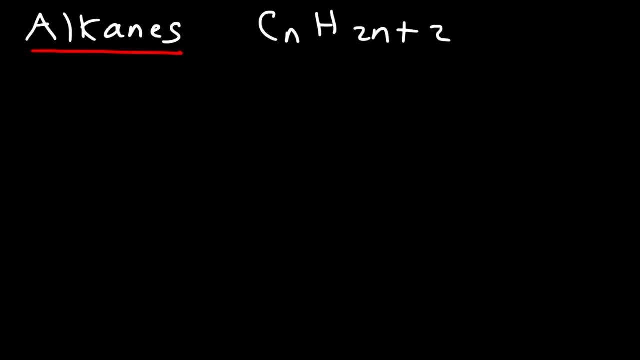 The general formula for an alkane is CnH2n plus 2.. The general formula for an alkane is CnH2n plus 2.. So the first example is C1H4.. So this is known as methane. 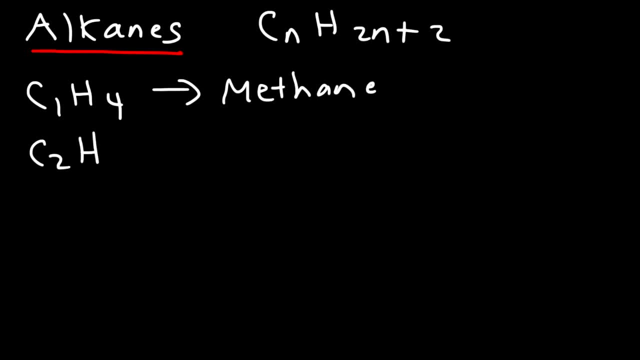 Next we have C2H6, and this is called ethane. C3H8, this is propane. Now, in most organic chemistry classes you need to know the first 10. So up to C10.. C4H8, if you have four carbons is going to be called a butane. And C5H12 is pentane. C6H14, if you want to write it down, that's hexane. C7H16 is heptane, C8H18 is octane, C9H20 is nonane. 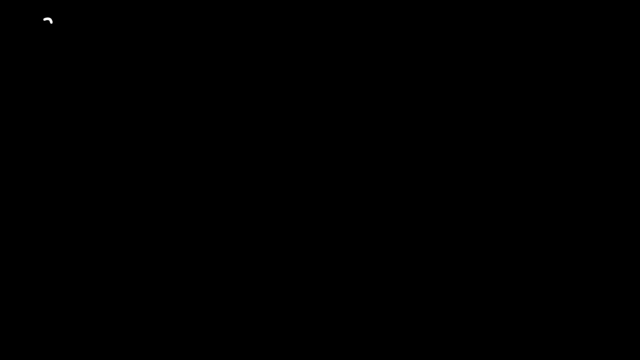 And C10H22 is decane. Now for those of you who need to know the first 10,. you need to know the first 10.. Now for those of you who need to know the first 20, here it is. 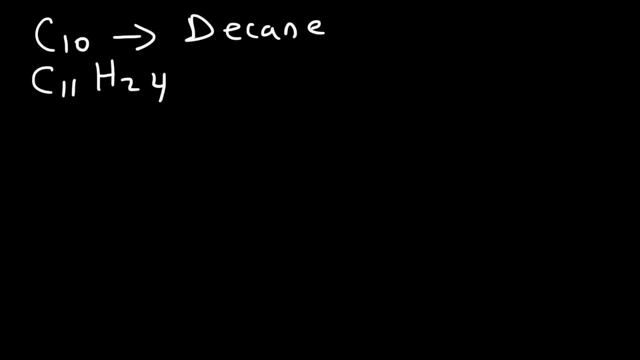 So C11H24, this is known as dodecane, And C12H26, that'sactually I take that back. C12 is dodecane And C11, this is undecane. C12 is dodecane. 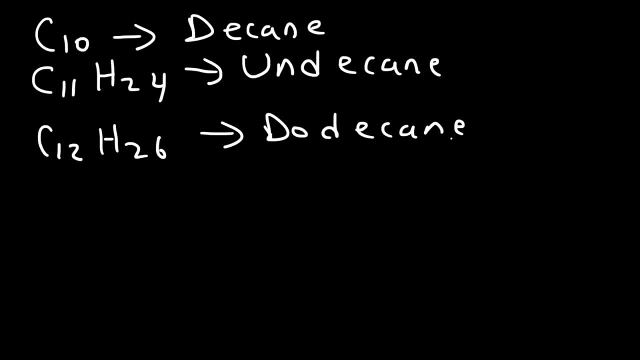 C13,, that's tridecane, C14,, tetradecane, C15,, pentadecane, C16,, hexadecane, C17,, heptadecane, C18 is octadecane. 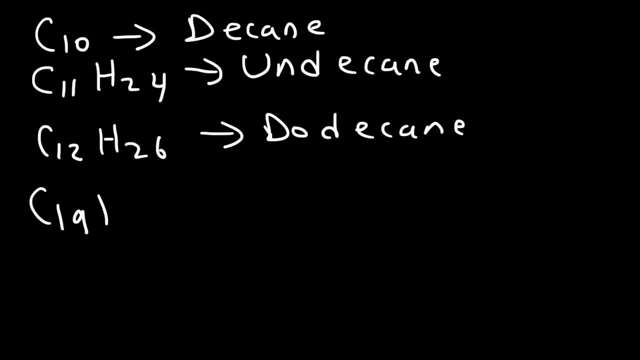 C19.I'll write this one down: H40, this is nanadecane. So you can see a pattern If you think about it: nana is 9, decane is 10.. If you add it, you get 19.. 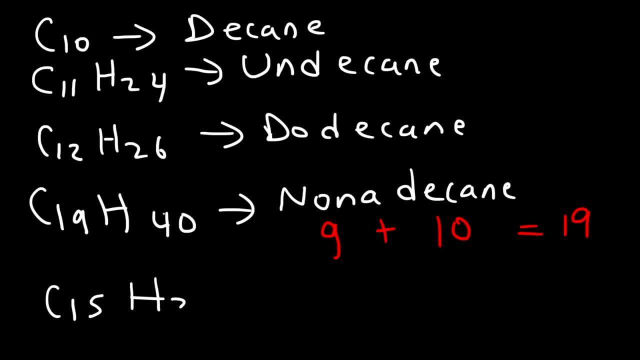 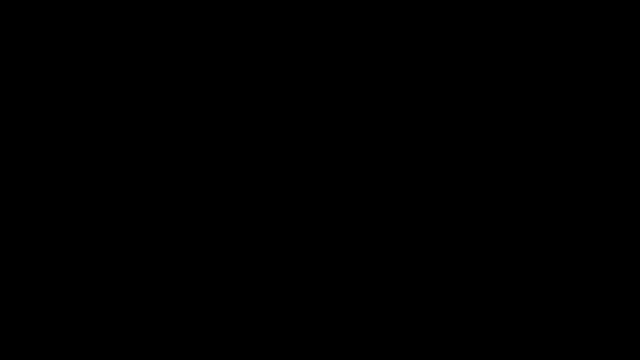 So, going back to C15H32, we said that was pentadecane. So penta, we know, symbolizes 5. Decane is 10.. 5 plus 10 will give you 15.. And the last one, C20.. 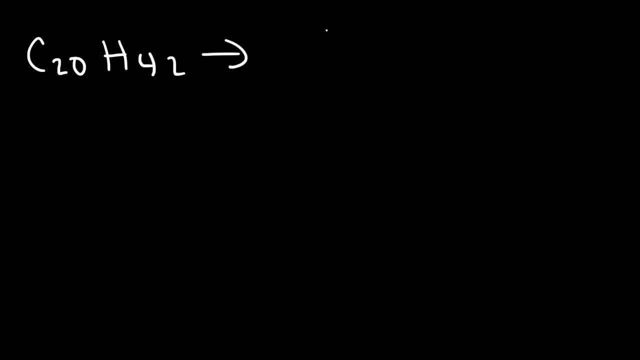 H42, this is called icosane, And I got no tricks for you for that one. Now let's talk about alkenes. Alkenes have the formula CnH2n if they only have one double bond or one pi bond. 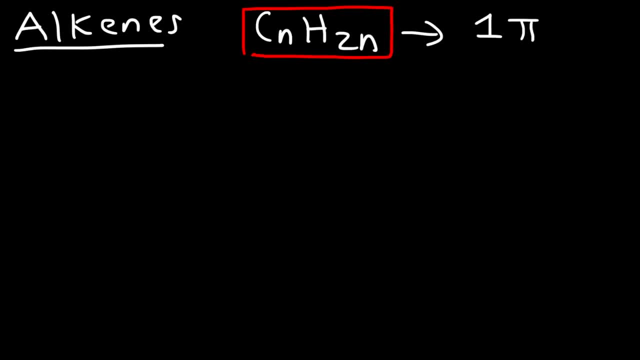 For each double bond that's found in the alkene, you need to decrease this by 5.. So if there's like two pi bonds, it's going to be CnH2n-2.. But if it only has one double bond, this is the general formula for an alkene. 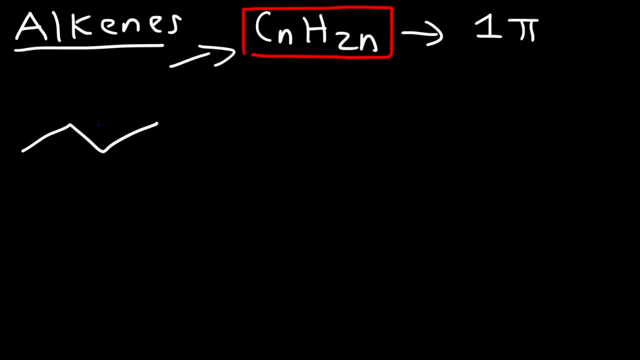 So, for instance, this is 2-butene, And if we were to draw out the structure, it would look like this: This is particularly trans-2-butene. If it was cis, the two methyl groups would be on the same side. 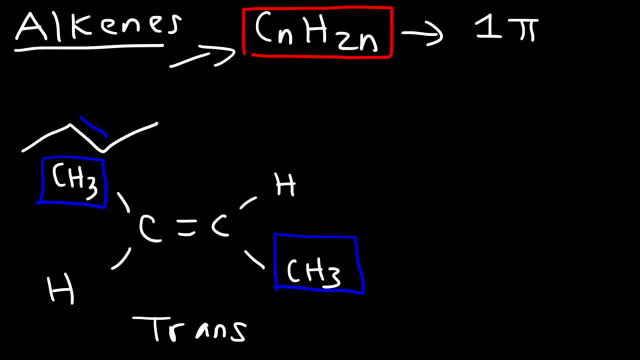 as opposed to opposite sides. Now, if you count the number of carbon atoms, 2-butene has 4 carbon atoms And there's 3 hydrogens here, 6, 7, 8. So it's C4H8.. 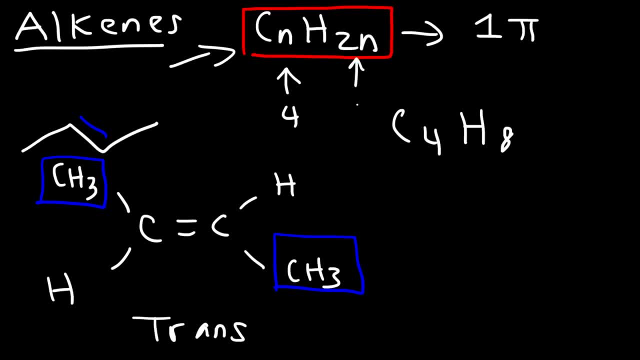 So in this case n is 4,, which means that 2n, or 2 times 4, is 8.. So alkanes have that general formula if they possess one double bond. It turns out that cycloalkanes 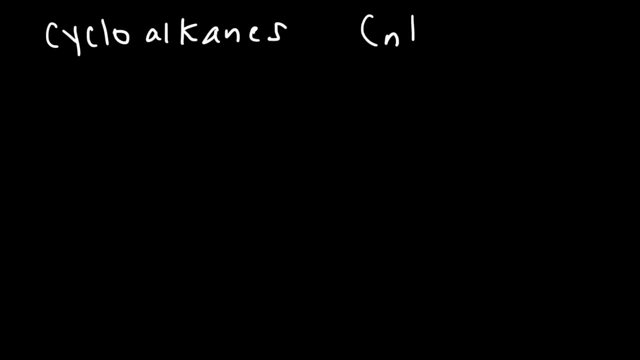 also have the same formula, CnH2n- if they have one ring. If they have two rings, then it's CnH2n-2.. So just keep that in mind. This is for one ring and this is if they have two rings. 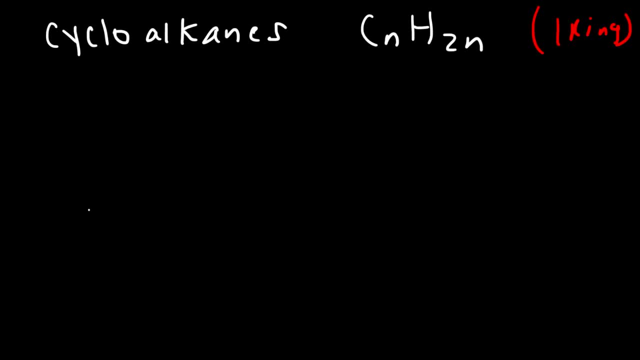 So a good example will be cyclopentane C5H10.. Now, carbon can only form four bonds, and every carbon atom is attached to two other carbon atoms, So there's only space for two hydrogen atoms on each carbon. 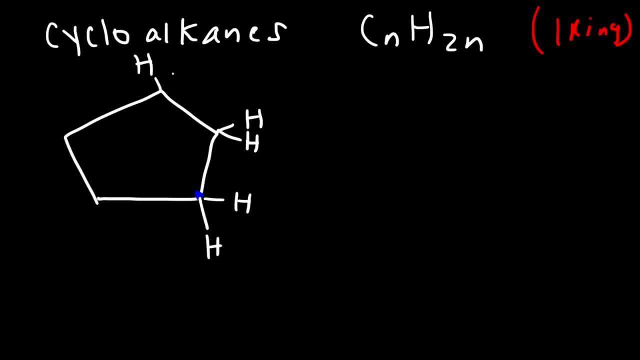 And so in this molecule we have a total of 5 carbon atoms and 10 hydrogen atoms, So it's C5H10.. Now let's compare this to a typical alkane such as pentane. Pentane is C5H12,. 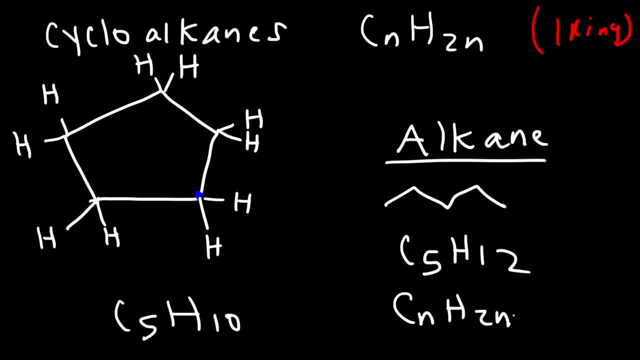 based on the formula CnH2n-2.. So alkanes have the maximum number of hydrogens per carbon atom, And so they're saturated. But any time you add a ring or a double bond you lose two hydrogen atoms. 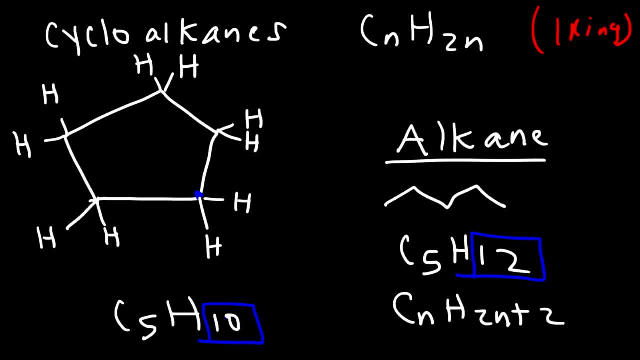 And so that's why alkanes are unsaturated. They don't have the maximum number of hydrogen atoms that they can have. So whenever you have a ring or a double bond, you lose two hydrogen atoms. If you have a triple bond, 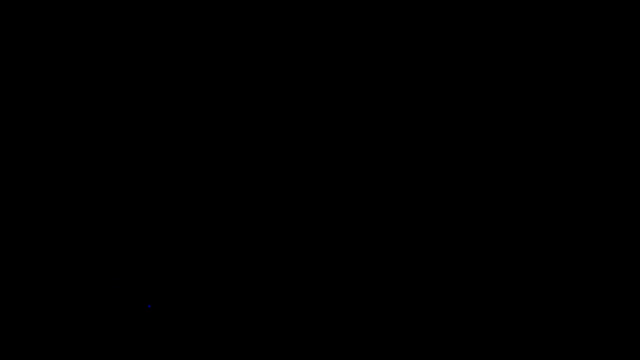 you will lose four hydrogen atoms. So in the case of alkynes, they have the chemical formula CnH2n-2.. CnH2n-2.. Assuming we have a molecule with one triple bond, For every triple bond you lose four hydrogen atoms. 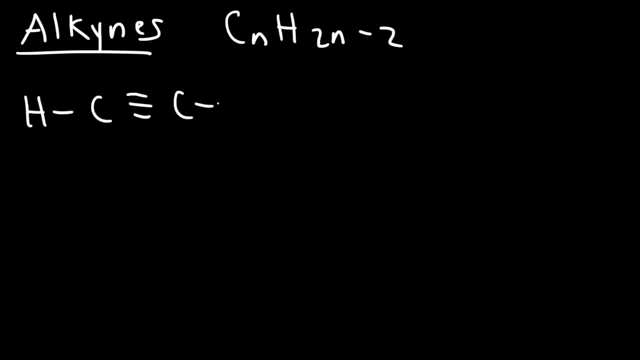 So let's look at acetylene: This is C2H2.. And if we compare it to ethane, which has the same number of carbons, this is C2H6.. So notice that the difference in the number of hydrogen atoms is four. 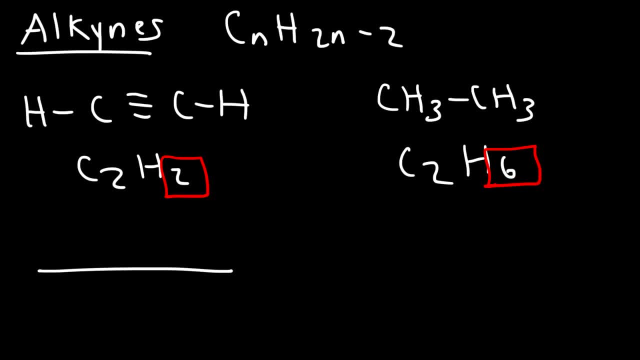 So let's look at another example. This molecule is called 2-butyne. If we draw it, it looks like this: So it's C4H6. Whereas if you compare it to the alkane butane, 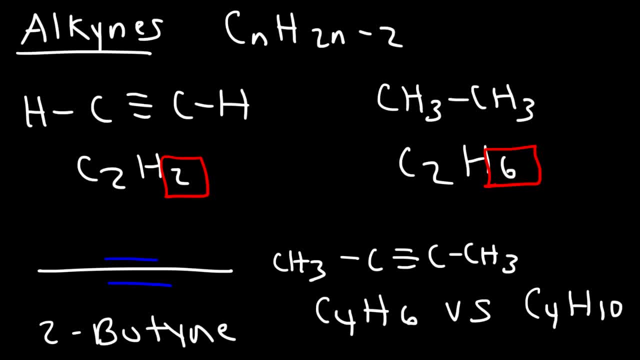 which is C4H10,, you'll see that there's a difference in four hydrogen atoms. So any time you introduce a double bond or a ring, two hydrogen atoms will be lost, And if you introduce a triple bond, four hydrogen atoms will be lost. 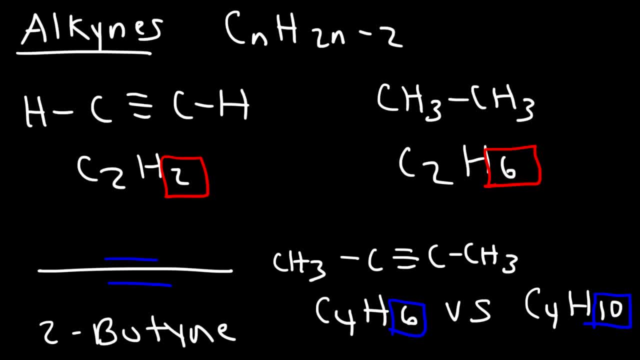 And so I want to give you a basic introduction into hydrocarbons, And they're basically molecules that contain just carbon and hydrogen in it. So that's all I got for this video. Thanks for watching, And I guess I'll see you in the next video. Thanks for watching. 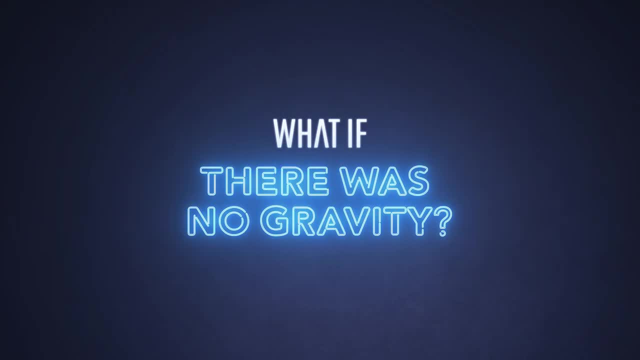 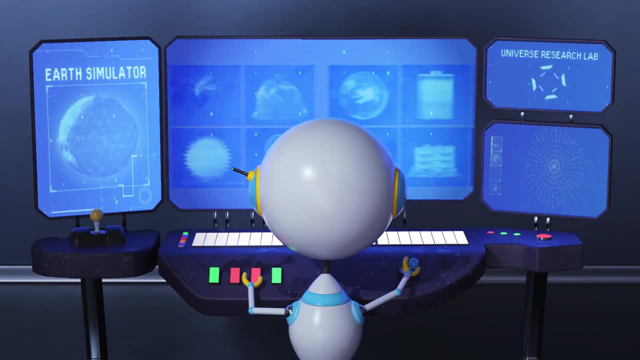 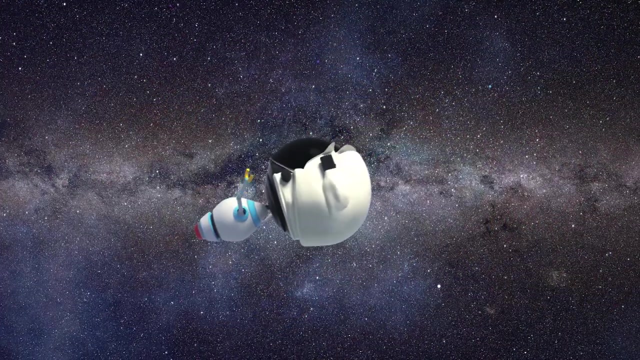 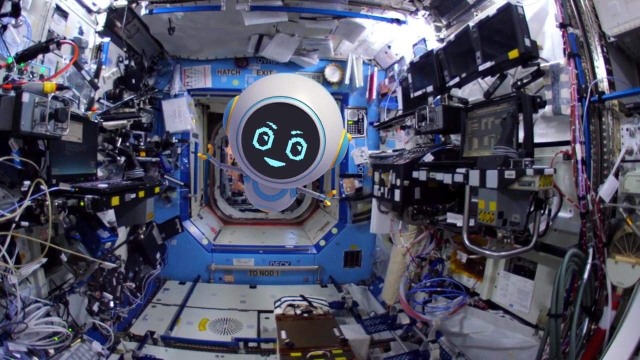 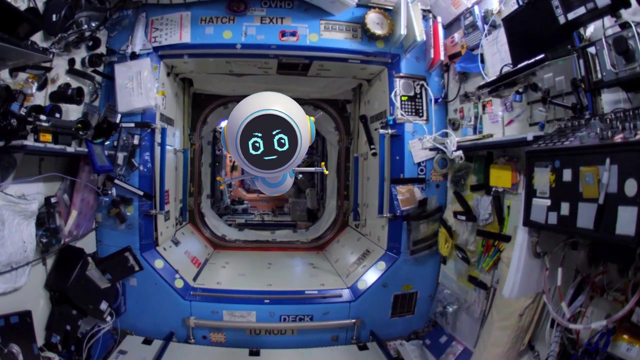 Hmm, Okay, what's happening today? Gravity, That's not a problem for me. The astronauts on the International Space Station don't worry about gravity either. If I want to study gravity, I should go to Earth. I know just who to call. 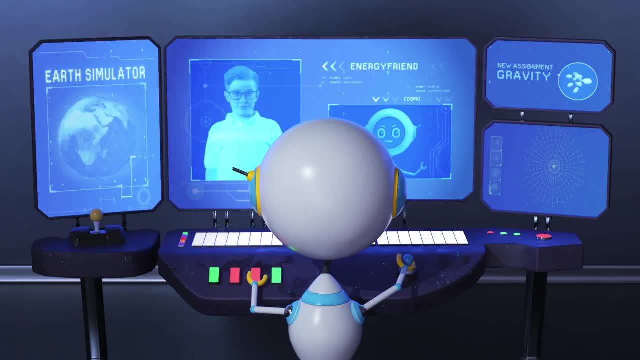 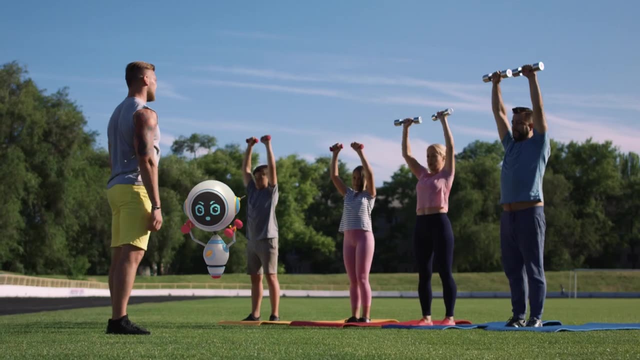 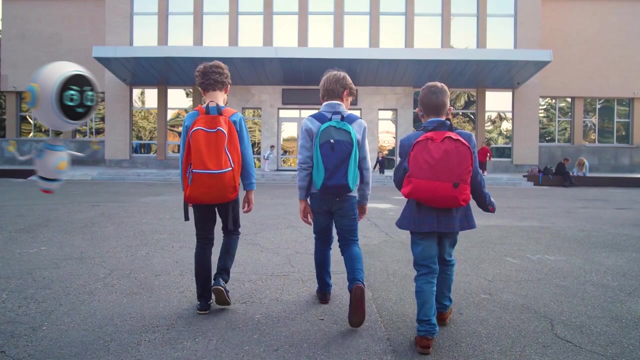 Hey energy friend, Can we talk about gravity? Of course, Gravity is an invisible force that holds everything together. Objects of greater mass have greater gravity and a strong pull. Gravity is the reason why Earth orbits the sun and why it can walk on Earth without floating in the air. 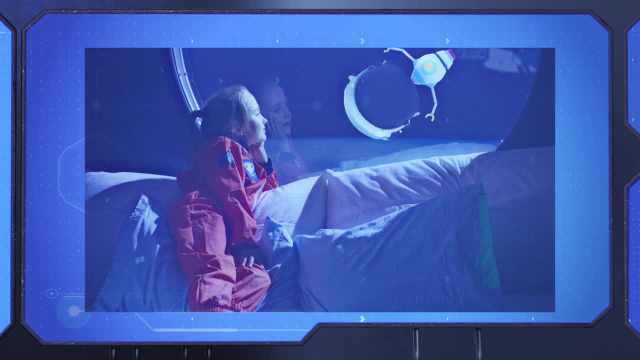 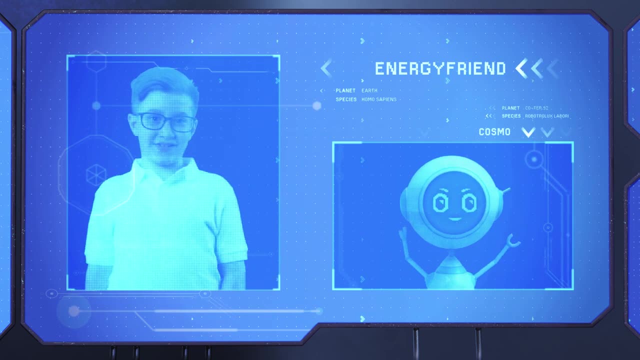 Okay, I've always wanted to float like an astronaut. Could you run a simulation and see what would happen if Earth had no gravity? Of course, What's the worst that could happen. I don't like the sound of that. but Start the simulation. With no gravity, your body would change, how your bones grow. Astronauts lose at least 14% of their bone strength during a six-month stay in space On Earth. gravity is the most important thing. Gravity naturally causes blood to flow into your legs and feet.